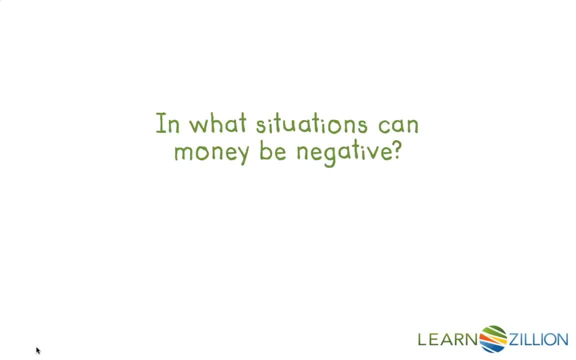 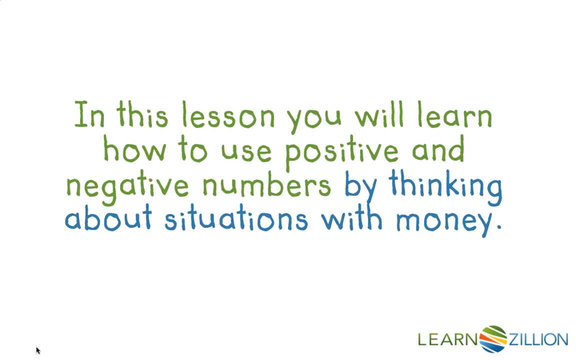 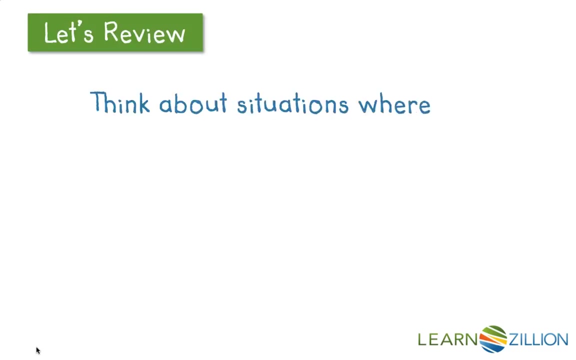 In what situations can money be negative? In this lesson, you will learn how to use positive and negative numbers by thinking about situations with money. Let's review. Think about situations where you have either spent money or lost it. In both cases, you don't have it anymore. A common mistake: Spending money. 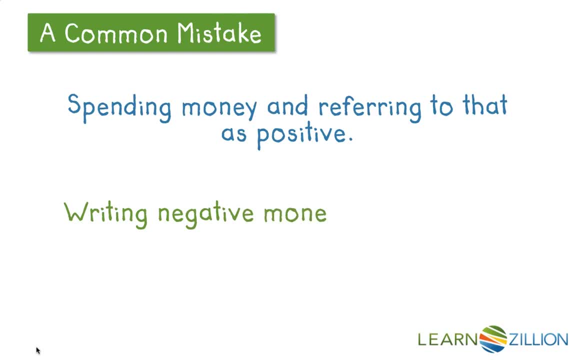 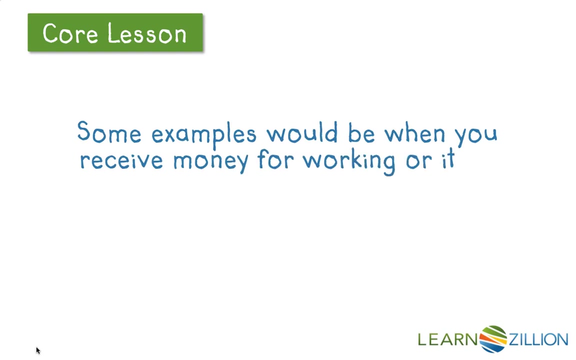 and referring to that as positive. Writing negative money as dollar sign. negative four instead of negative dollars: sign four. So think about times when money is positive. Some examples would be when you receive money for working or it's a gift, It's money that you actually have. My 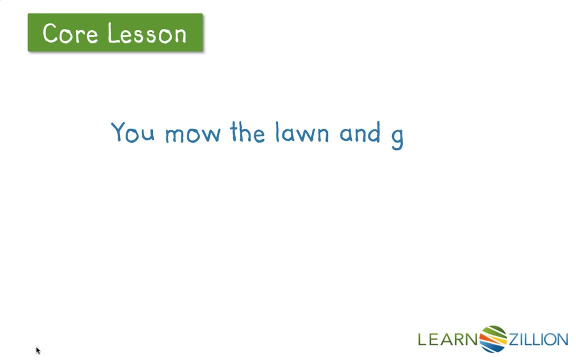 So say you money for work or it's a gift, It's money that you actually have. So say you money for work or it's a gift, It's money that you actually have. So say you mow the lawn and you get ten dollars. that would be positive, you get money for. 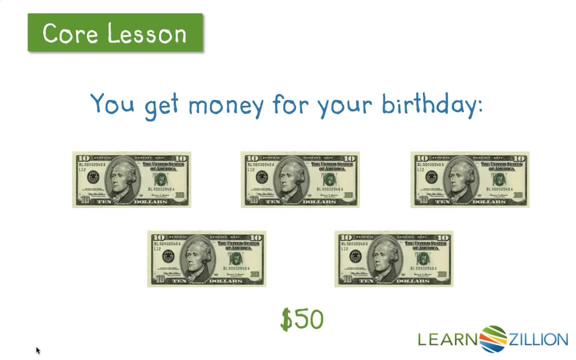 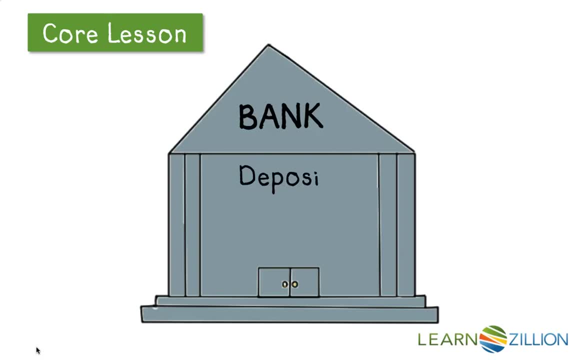 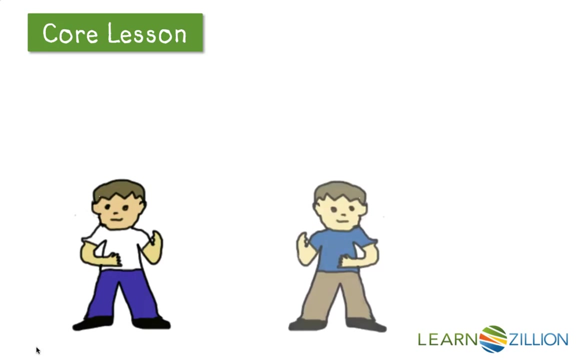 your birthday, you got fifty dollars. that would also be positive. sometimes people keep money in a bank. in a bank you deposit your money and you deposit it into a savings account or checking account. money that you have in the bank is positive money. now what about when money is negative? here two boys are. 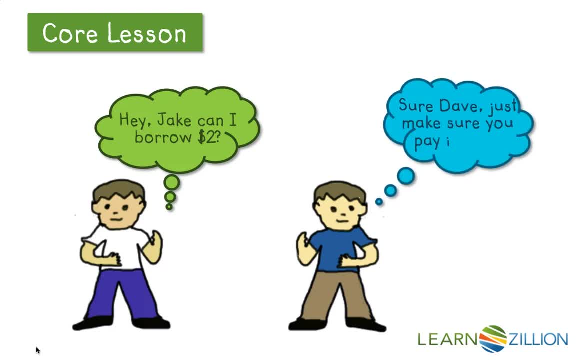 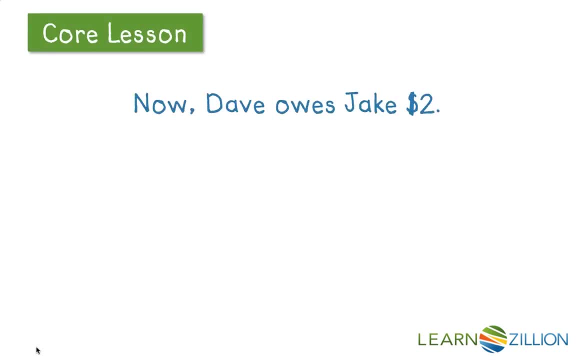 talking about borrowing money. Dave wants to borrow money from Jake, so now Dave owes Jake two dollars, so that would be considered negative two dollars. suppose you go to the mall and you buy a shirt. it costs fifteen dollars. we would write that as negative fifteen dollars, because it's money you spent. you don't have it anymore. suppose you buy a car. it's 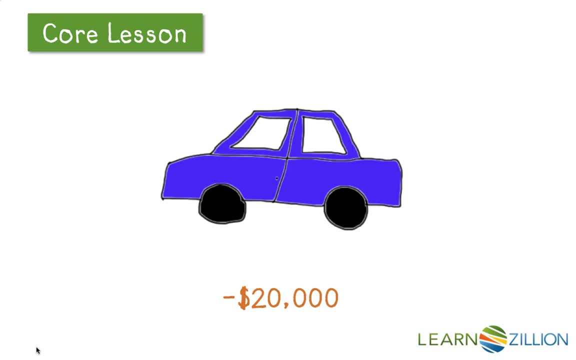 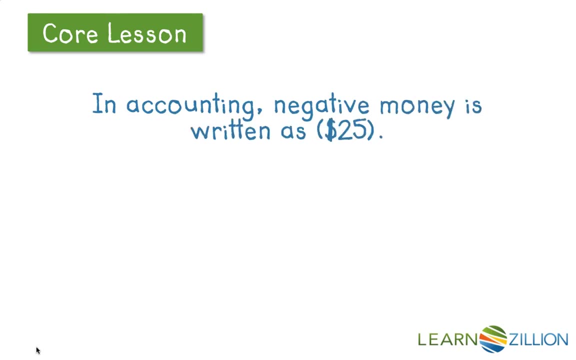 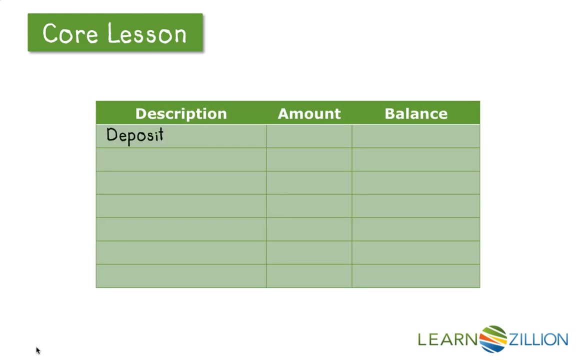 twenty thousand dollars. you're spending money, so it would be negative twenty thousand dollars. in accounting, negative money is written with the money inside parentheses. this is the same as negative twenty five dollars. so let's look at a bank account. you make a deposit into your bank for a hundred.